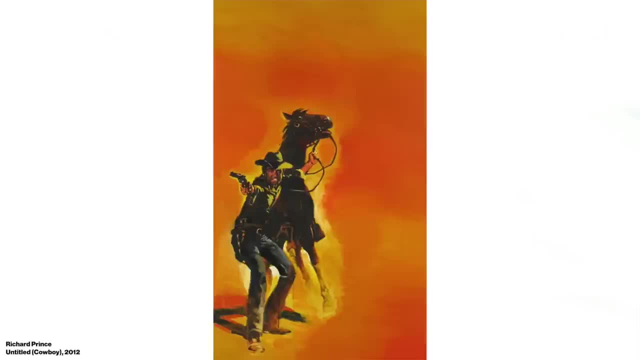 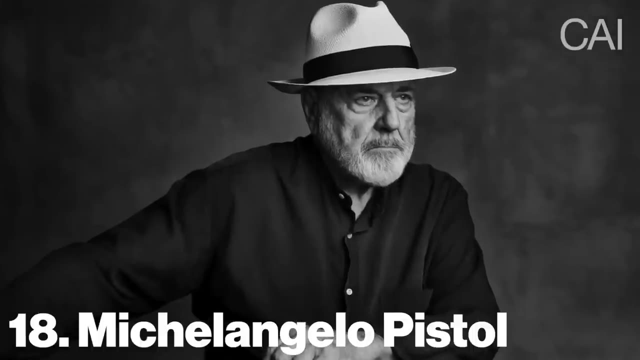 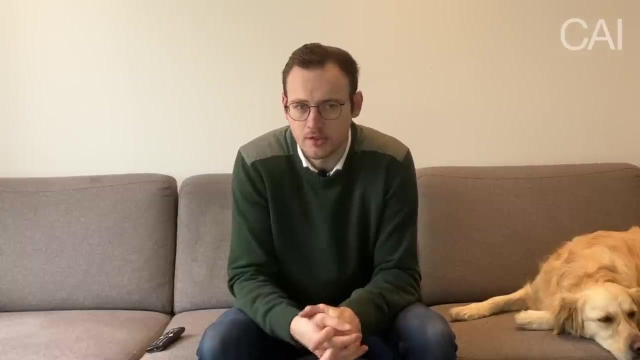 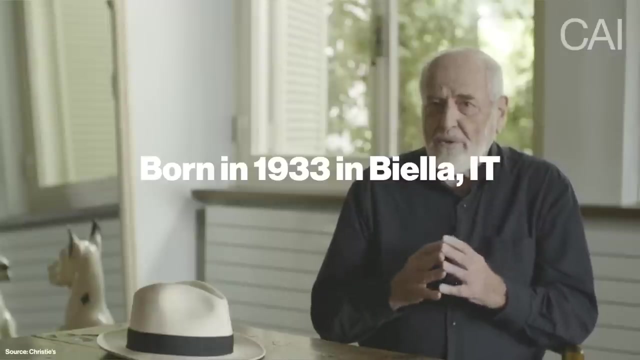 consists of subjects with an almost mythical status, such as cowboys, bikers, celebrities and paintings of nurses. although he is best known as a prominent figure for art povera and a representative of conceptual art, michelangelo pistoletto was also very influential as a painter. born in 1933 in biella, italy, pistoletto achieved international recognition. 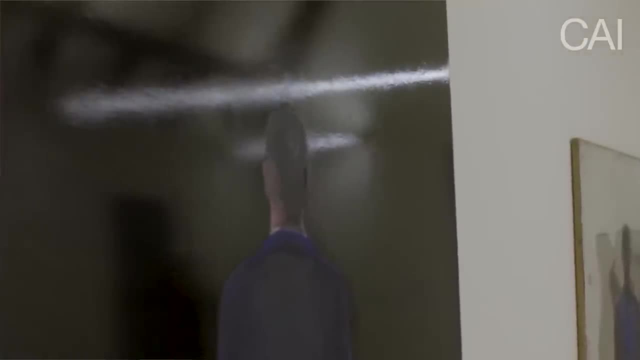 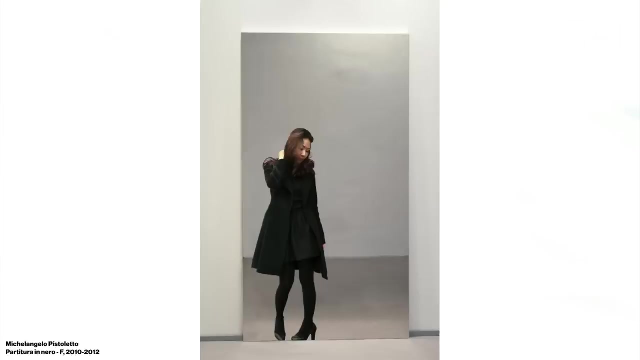 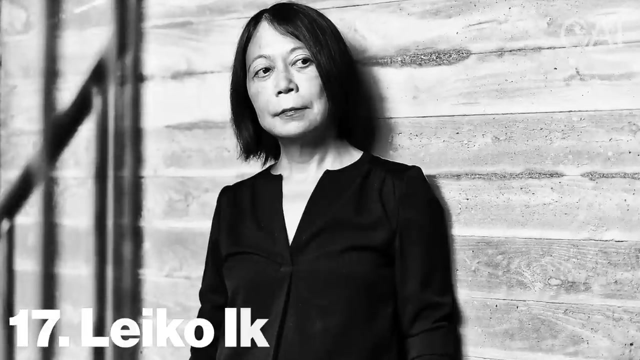 with his mirror paintings at the start of the second half of the 20th century. using metallic paint on canvas or polished steel, pistoletto plays with the notion of the mirror and reflection, bringing the viewer and his or her environment into the painting itself. bon lord. 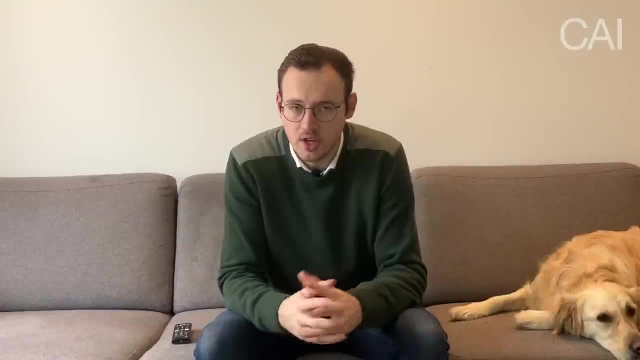 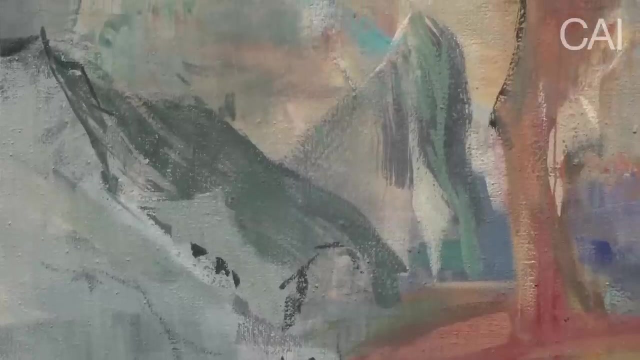 born in 1951 in japan and residing and working between cologne and berlin in germany, laiko ikimura is also a renowned painter and sculptor. it is to say, she is mainly a painter, but is also active as a draughtswoman and a sculptor since 1981, and also as a 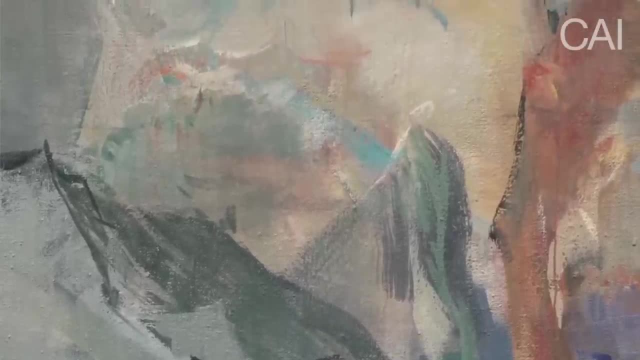 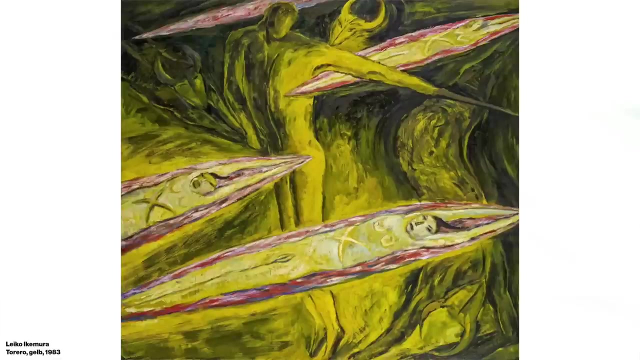 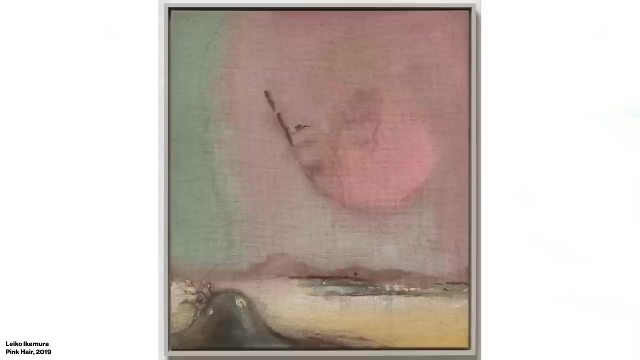 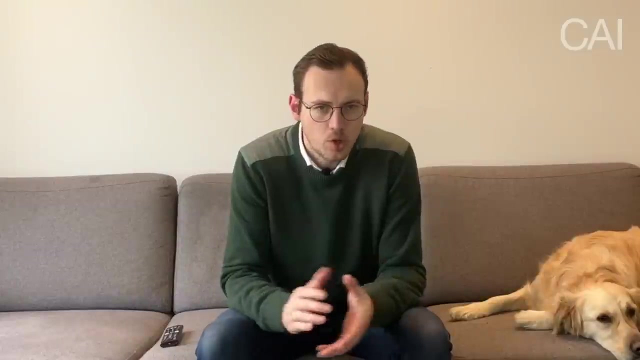 photographer recently. herbuat is marked by a mysterious aura residing in her mystical landscapes and obscure portraits. Ikumura balances between abstraction, expression and figuration as her guideline. In doing so, the Japanese contemporary artist examines gender, war and religious issues. Next, we have one of my personal favourites, Marlene Dumas, born in 1953 in Cape Town. 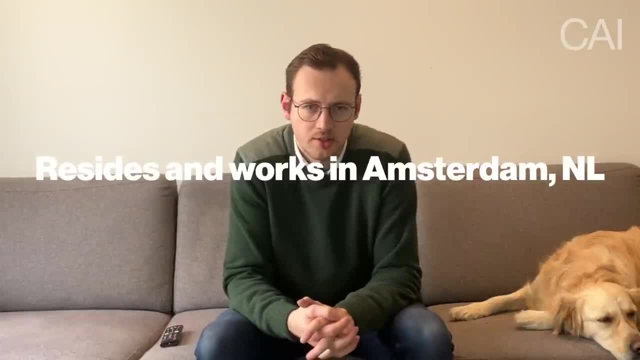 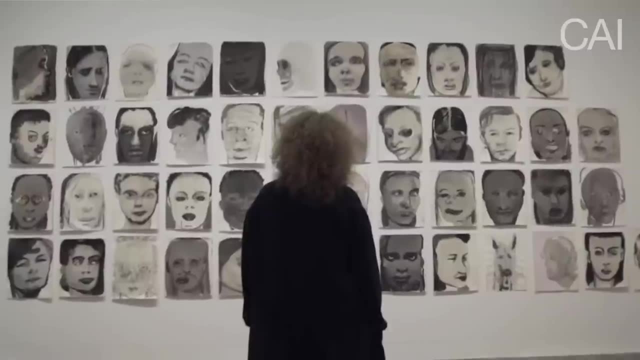 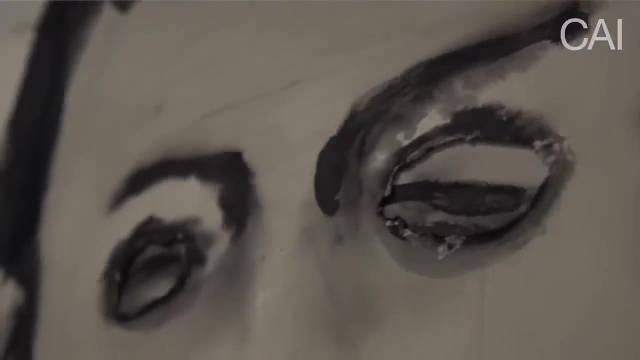 South Africa and residing and working in Amsterdam, the Netherlands. Dumas is known for her distinctive figurative language, sensually painted figures and often thought-provoking subjects. Dumas feverishly collects images from which she draws inspiration and, as a result, she merges political issues with personal experiences and art historical references. 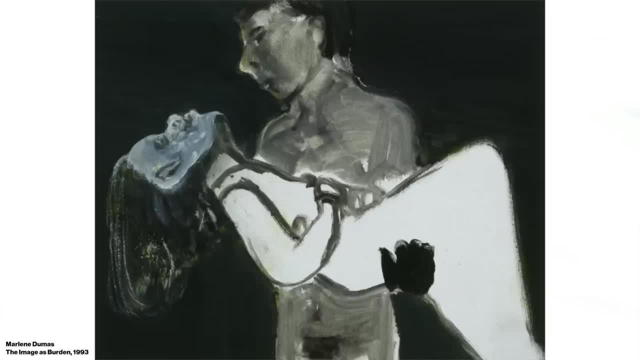 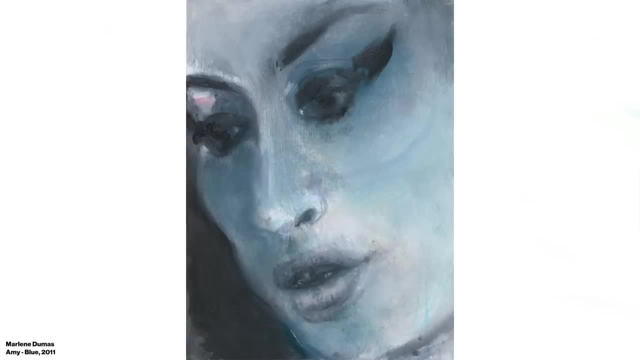 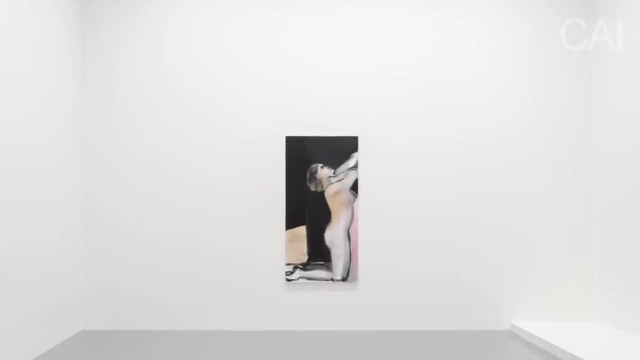 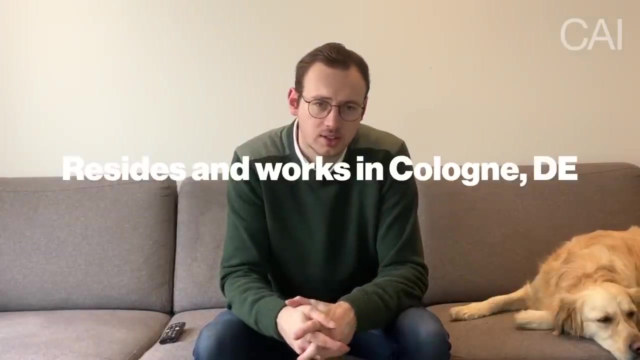 with a personal approach to the canvas, Being one of the most important painters of the broader movement of new European painting. themes such as segregation, politics, war and the cultural processes of objectification are examined in a personal yet universal manner. Albert Ullen, born in 1953 in Krefeld and currently residing in Cologne. 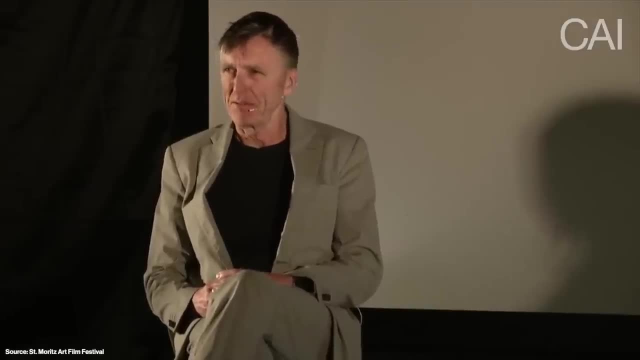 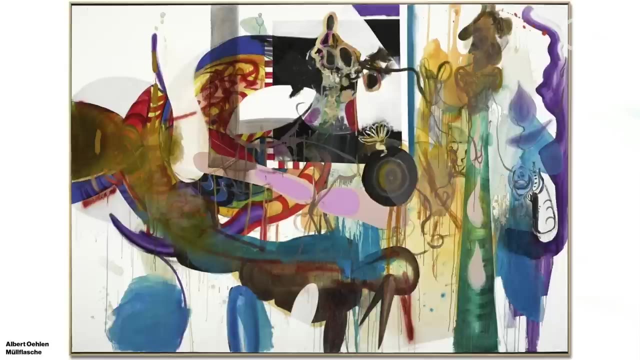 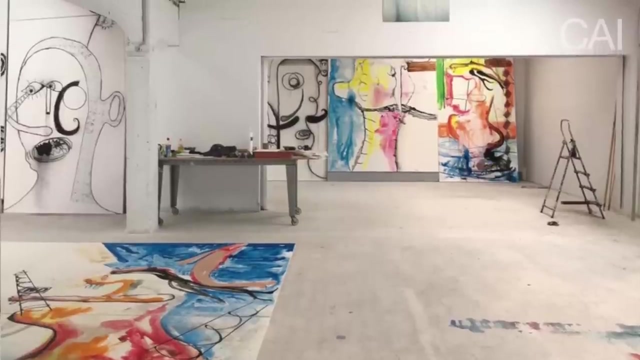 is a German painter marked by freedom and creativity. Ullen's oeuvre is characterised by expressionist brushwork, an écriture automatique and a history of abstraction and an ongoing quest for new extremes. In the 80s, Ullen became a dominant figure in Berlin and in the Cologne art scene. 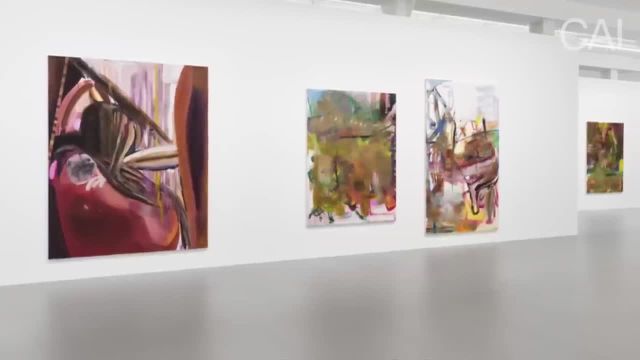 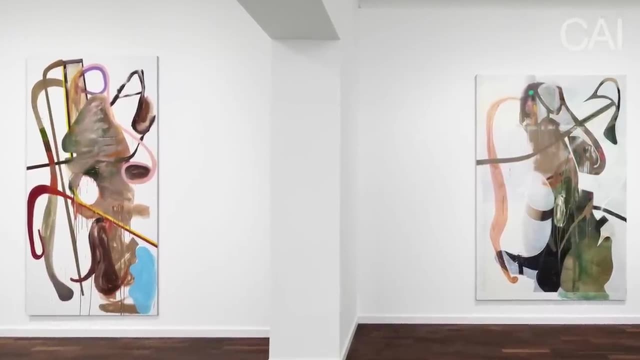 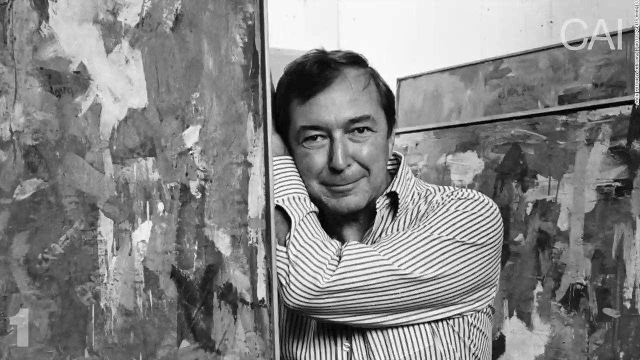 alongside the Neue Wilde, such as Martin Kippenberger or Werner Büttner, The German artist attempts to deconstruct the medium, investigating painting's most essential aspects, such as colour, the brushstroke as a gesture, motion and time. Jasper Johns, born in 1930 in Augusta. 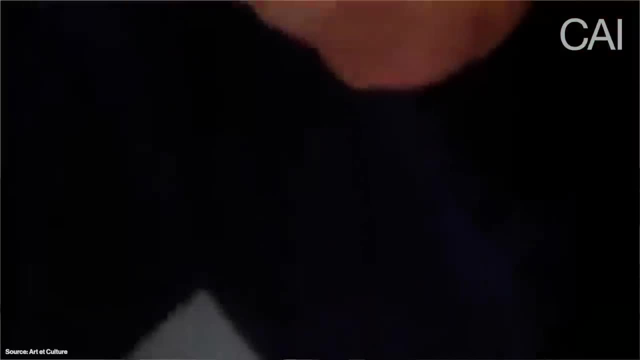 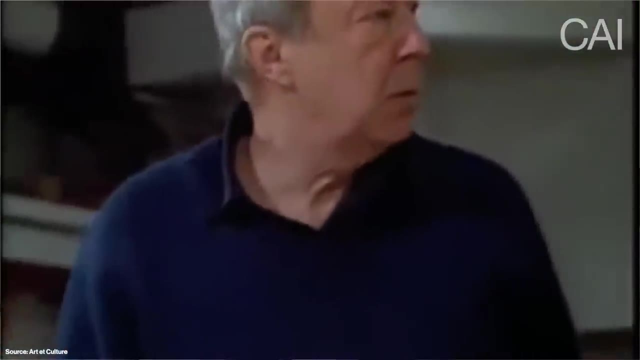 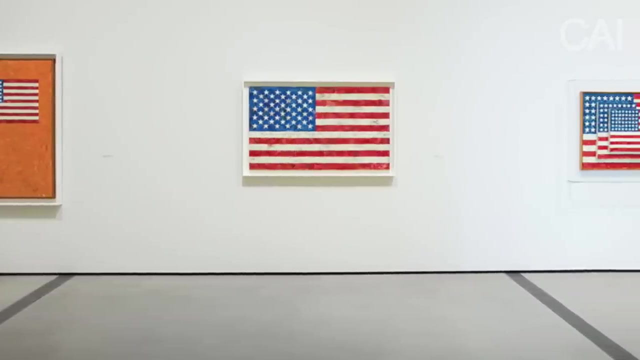 and currently residing and working in Sharon, Connecticut, is an American painter and the winner of the Golden Lion Award, a major recognition at the Venice Biennale in 1988. He is arguably best known for his iconic flag paintings, Hovering between abstract expressionism and pop art. Johns approaches the American flag in a 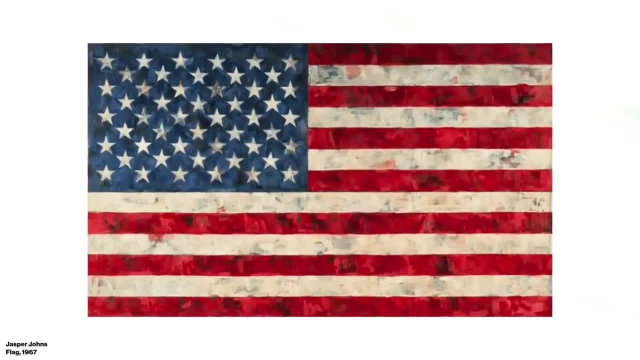 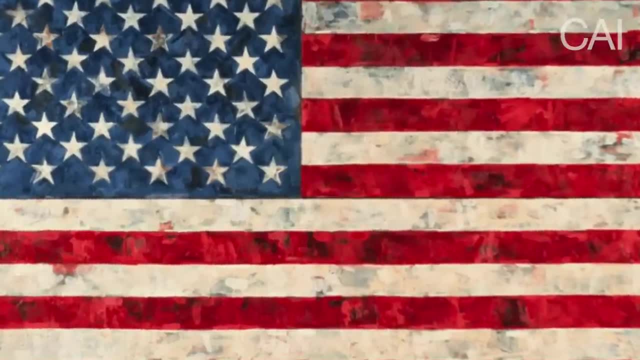 rather formalist manner effectuating the image's power. The stripes and stars are redefined as shapes arranging the picture. The image is a symbol of the American flag, a symbol of the American people, as a painting and as a statement. 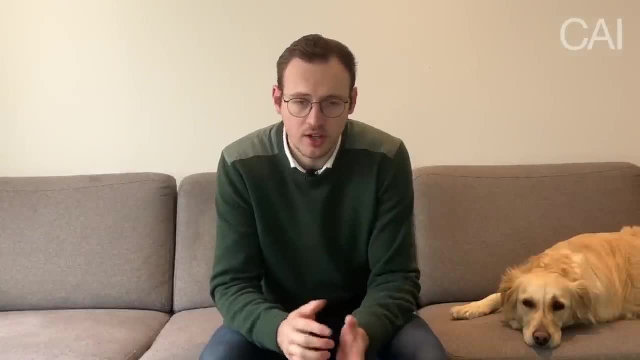 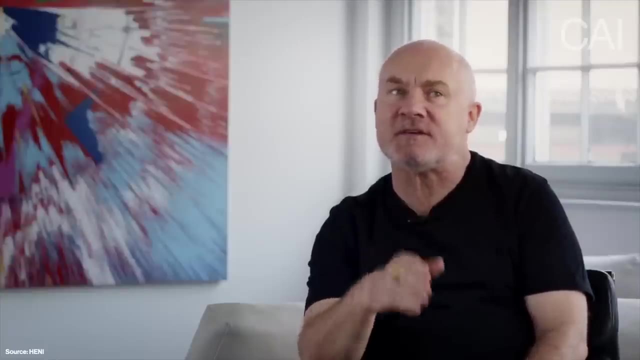 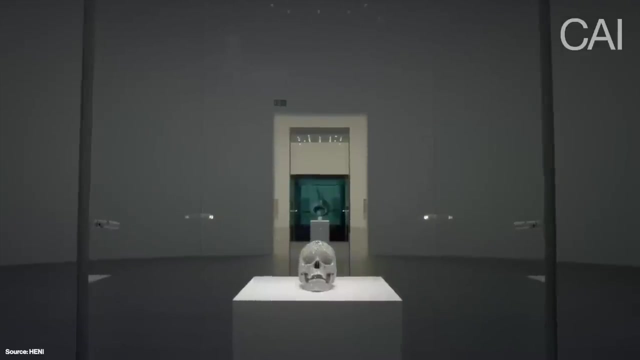 Born in 1965 in Bristol and residing and working in the English capital, London, Damien Hirst is one of the most popular and controversial artists of his generation. He rose to fame in the late 1980s with his often shocking sculptures pushing the boundaries of good art, good taste or simply the acceptable, but is also renowned. 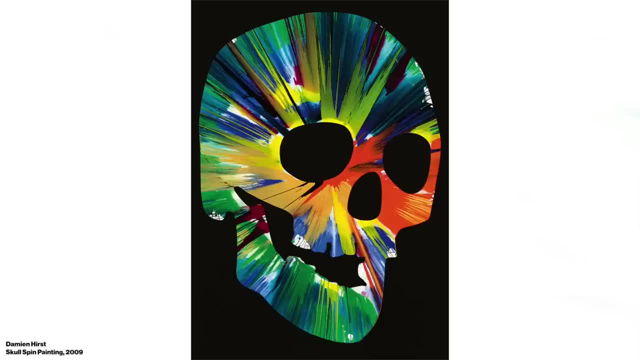 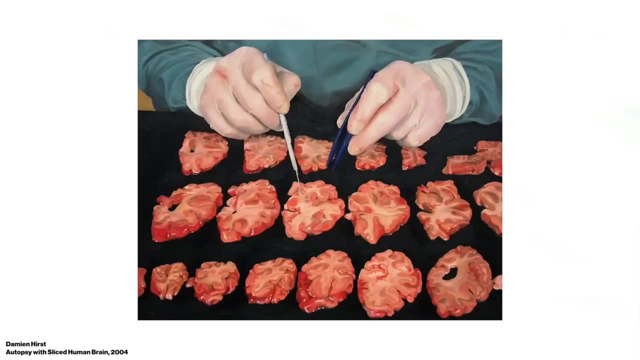 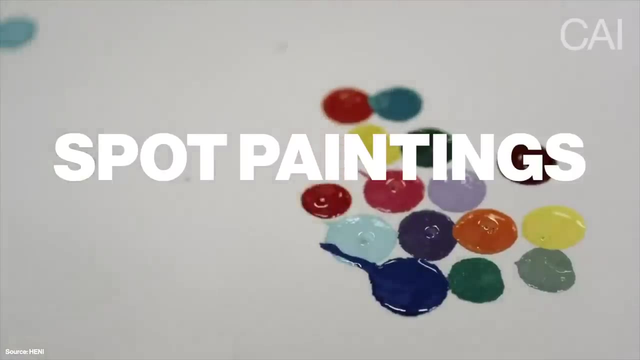 for his painterly practice, depicting dots, butterflies, flowers, skulls and more. Hirst examines the complex relationships of religion versus science, art and beauty or life versus death. His serialised paintings of multi-coloured spots challenge belief systems and the uncertainties of the human condition and experience. 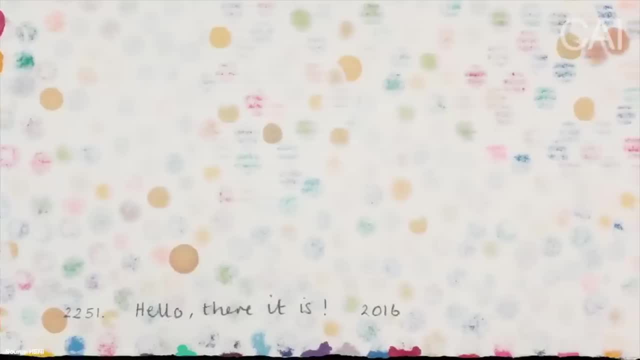 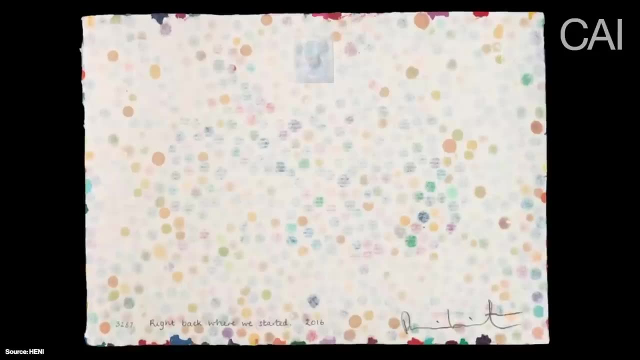 His Pot Paintings. a series that originated in the mid-1980s and continues up to this very day, with over a thousand works of art, is one of the most popular works of art in the United States. Hirst's collection of over a thousand pieces to date is an ongoing search to paint as a machine. 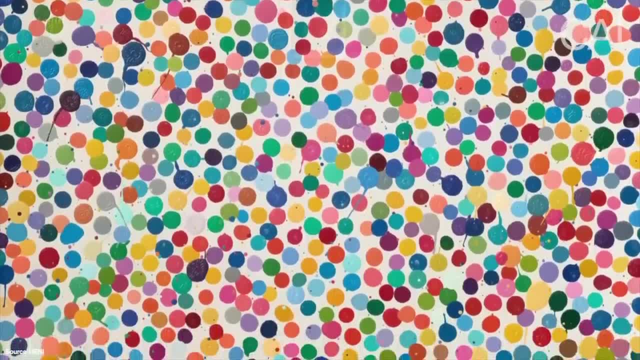 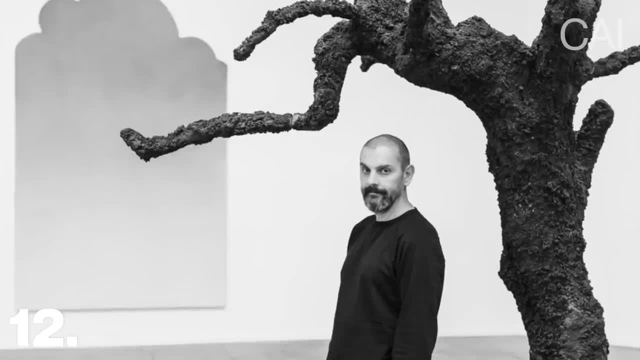 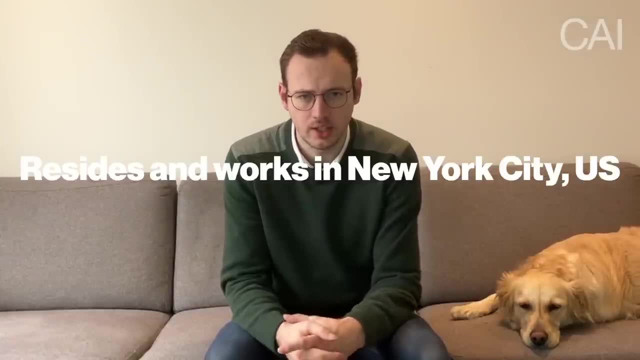 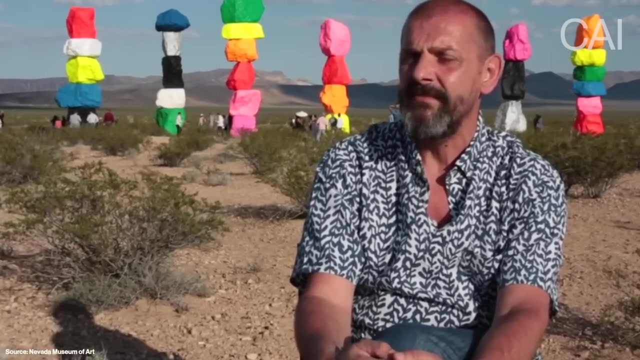 but allowing subtle imperfections to dictate the overall feeling of the painting, making them both calming and unnerving, beautiful and ordinary. Born in 1964 in Brunnen, Switzerland, and currently residing and working in New York City, Ugo Rondinone is one of the most important artists of his generation, occupied with painting but also. 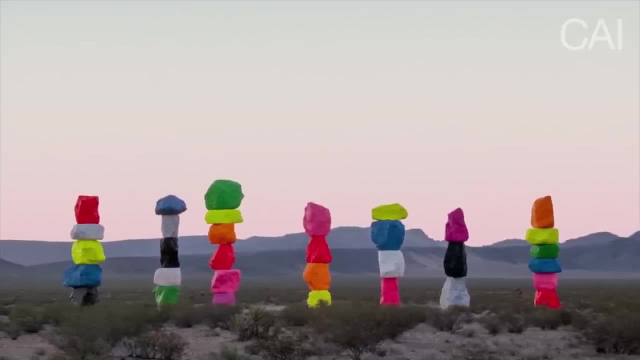 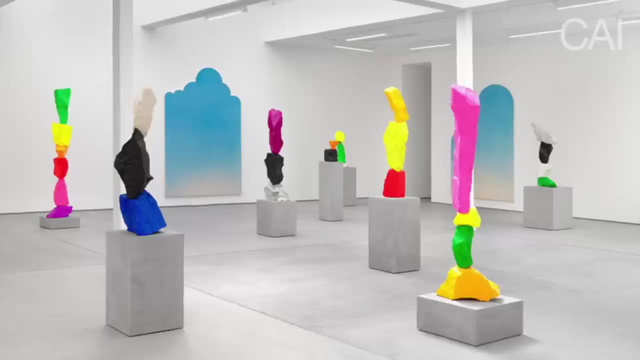 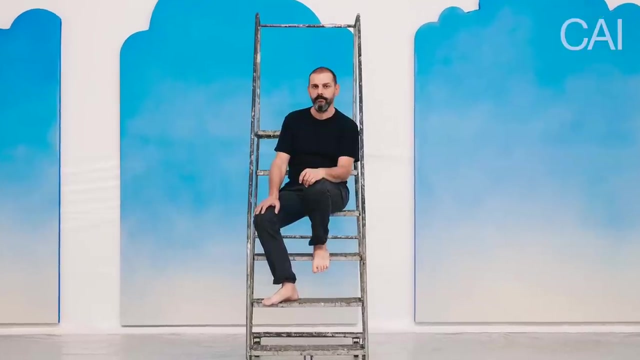 large-scale drawings, sculptures and installations. Throughout those various disciplines, and in particular with his almost psychedelic paintings, Rondinone explores the relationships between opposites. Think of night versus day, artificial versus real or even euphoria versus depression. His neon-hued mandala paintings are arguably one of. 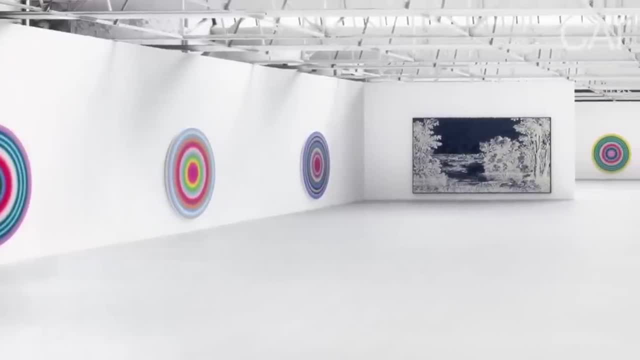 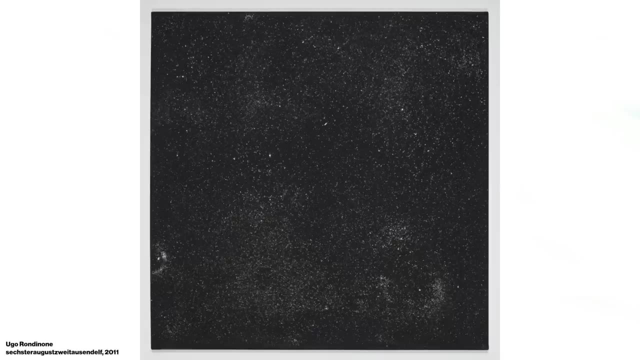 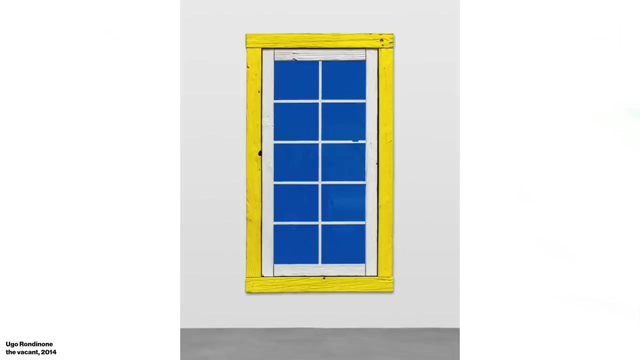 his most iconic series of works, alongside his coloured stacked rock sculptures. Still, when it comes to his painterly practice, there is much more to discover. Think of the abstracted landscapes, the irregularly shaped canvases resembling clouds, monochromes and even trompe l'oeils with a sculptural quality. 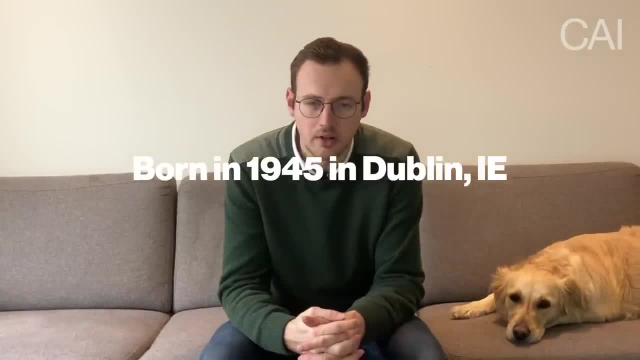 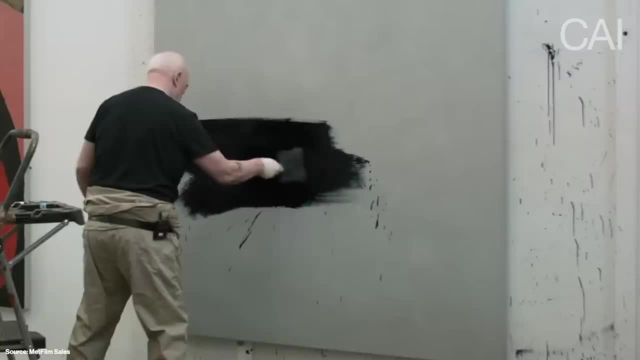 Sean Scully, born in 1945 in Dublin, Ireland and residing and working in New York City. Scully is one of the most important painters of the post-war era and is best known for his large-scale abstract paintings of vertical and horizontal shapes and planes. 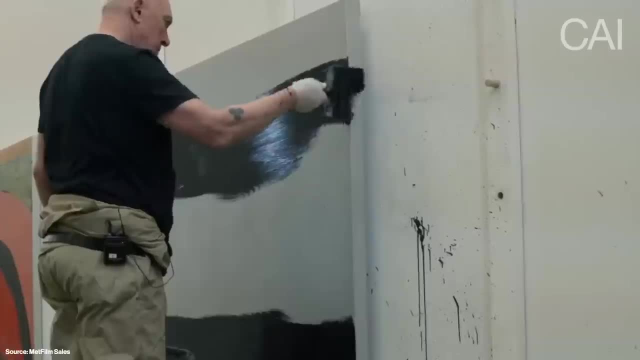 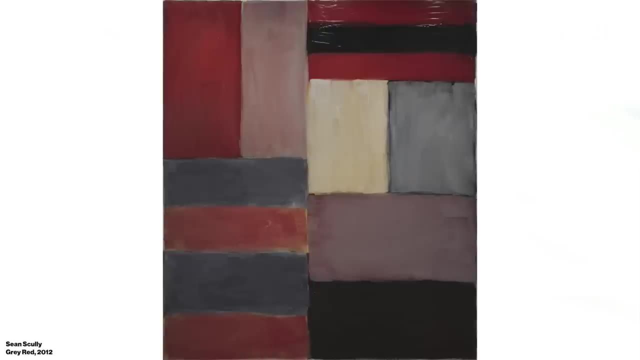 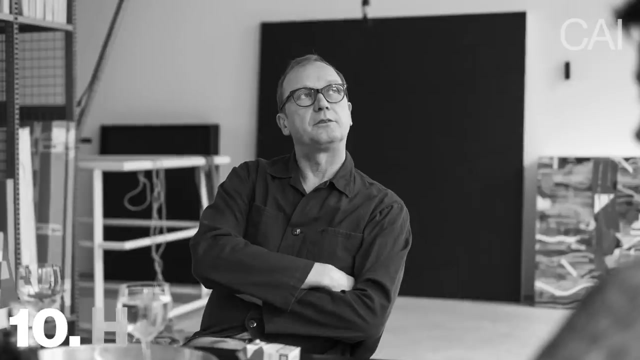 A synthesis of the dominant American abstraction and Scully's European heritage results in a personal style dominated by geometrical forms. Vertical and horizontal blocks connect, as the painting is filled with gestures and tangible emotions. Simon Zobernig, born in 1958 in Mauten, Austria. 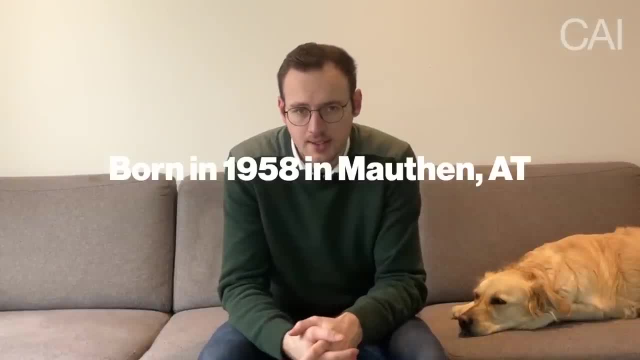 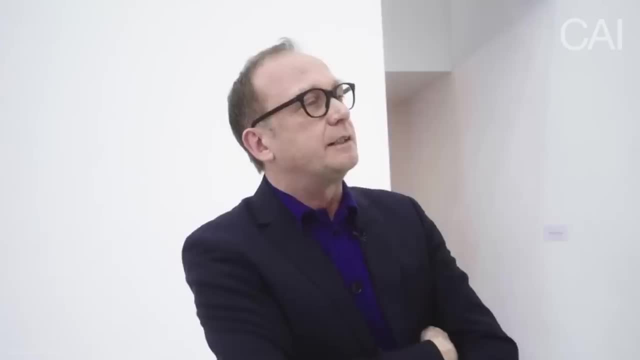 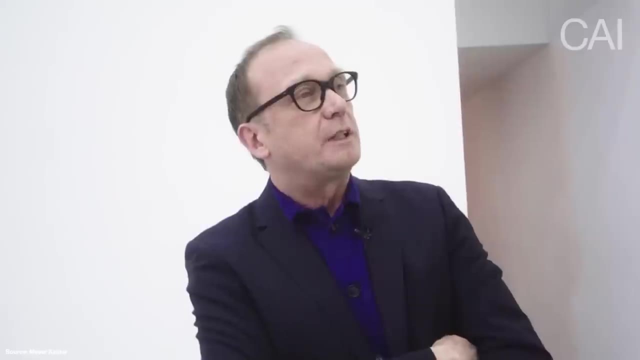 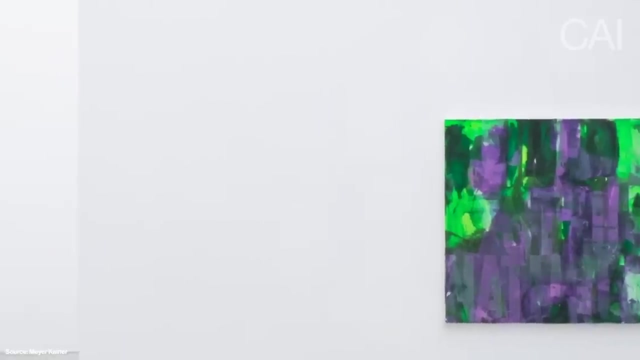 Simon Zobernig, born in 1958 in Mauten, Austria, And currently residing and working in Vienna. The Austrian artist defies categorization, implementing an extensive array of media in his artistic practice, such as architectural interventions, installation, film, video, sculpture and, of course, painting. 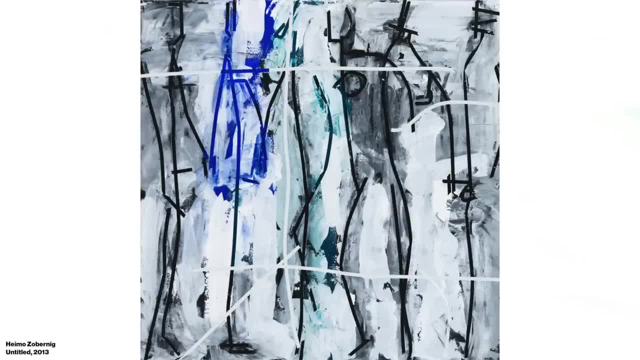 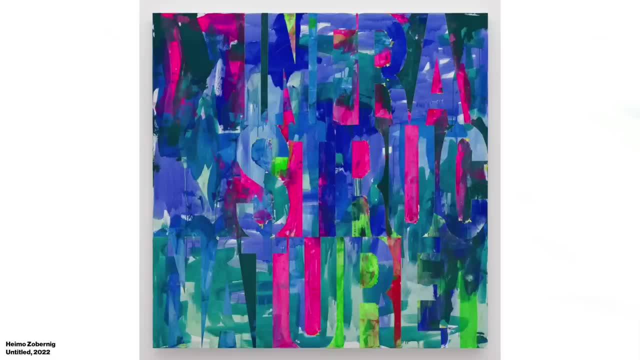 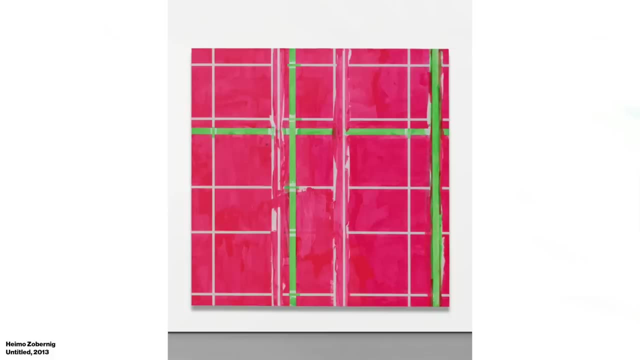 His oeuvre is marked by an interrogation of the formal language of modernism. Think of motifs such as the monochrome, the grid or geometric abstraction, to just name a few. Even more, Zobernig tends to go a step further and examines how his art is presented or framed. 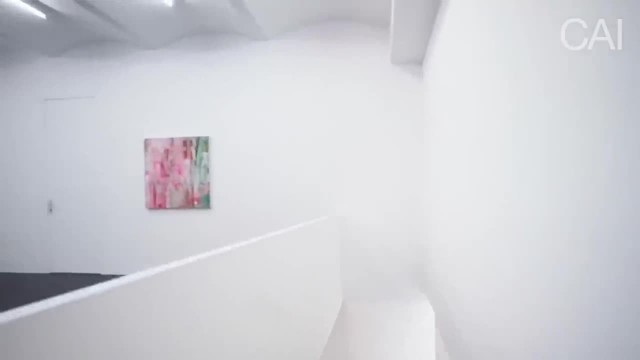 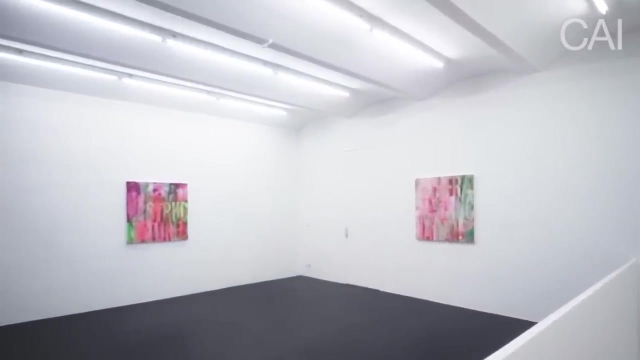 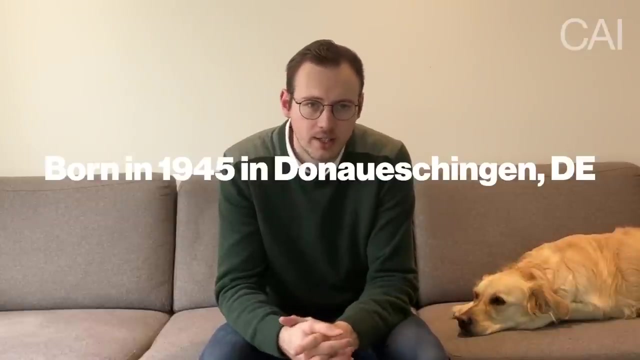 physically, but also conceptually In doing so. Simon Zobernig questions traditional gallery, architecture and art-historical and ideological concerns. teil 2: Anselm Kiefer asked lost questions. Who was born in 1945 in Don omega in Paris? 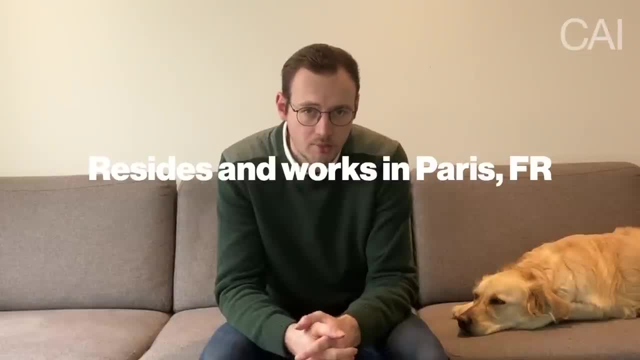 Anselm Kiefer, who was born in 1945 in Don chang, Mac оф, Mainfeedung, Werat 집, and currently residing and working in Paris. Do you know, Having grown up between the ruins of the Second World War, Kiefer's oeuvre is marked by Germany's 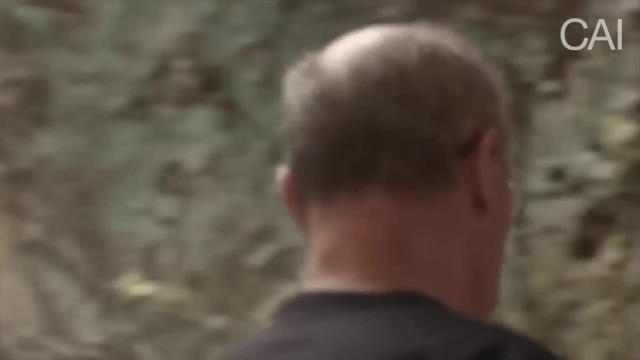 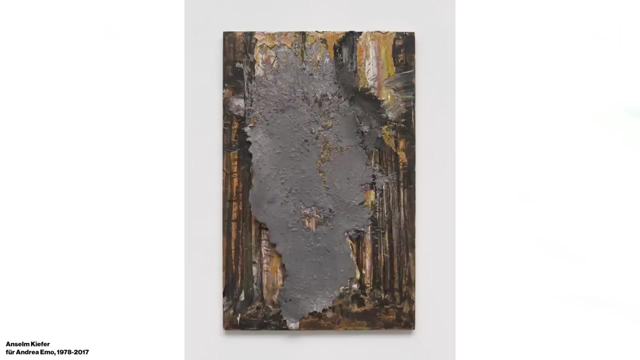 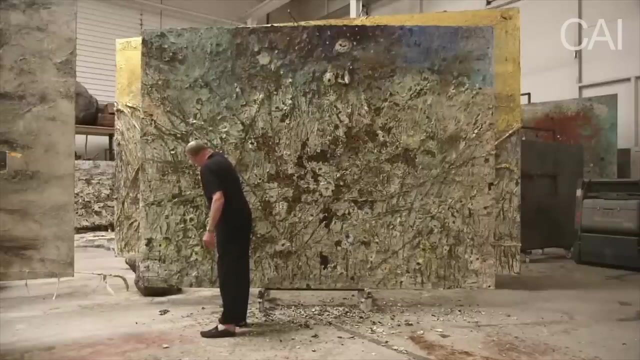 post-war identity into a broader movement of new European painting. Kiefer's paintings are marked by a rough surface, sculpting his paintings with metals and even implementing found objects. In doing so, Kiefer goes beyond reflecting historical events encompassing myth, spirituality and memory. 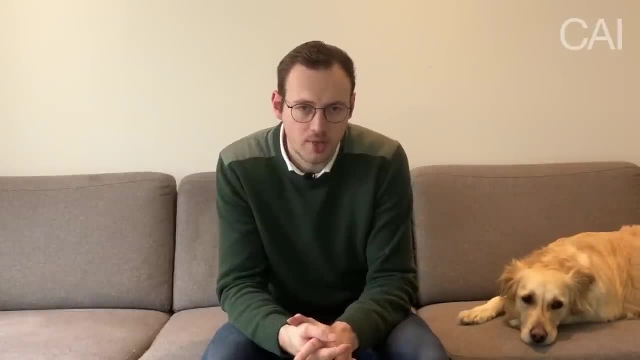 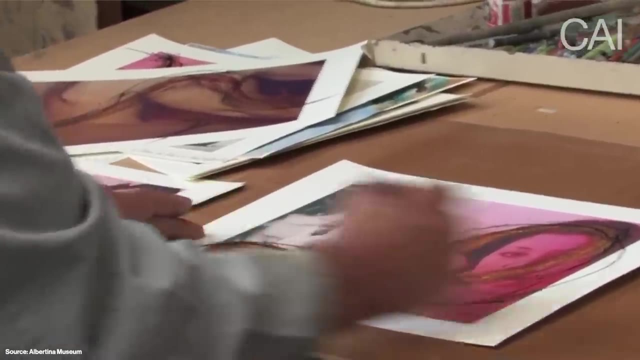 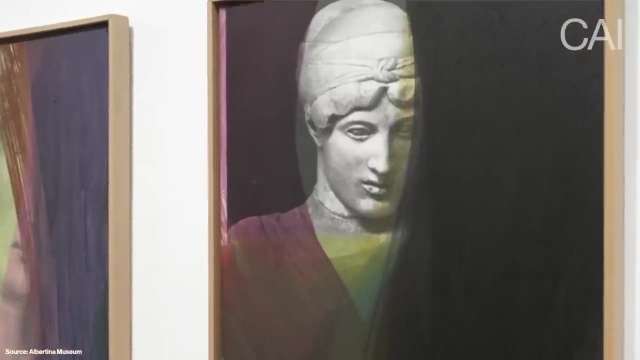 Born in 1929 in Baden, Austria, Arnulf Reiner currently resides and works in Vienna. Reiner achieved international recognition for his unique process of layering paint over photographic material. Marked by his use of appropriation, Reiner transforms existing artworks by painting. 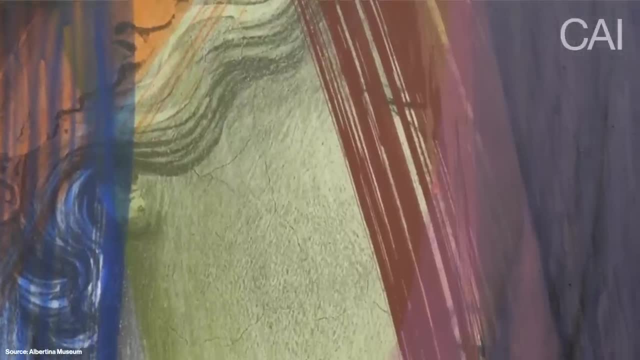 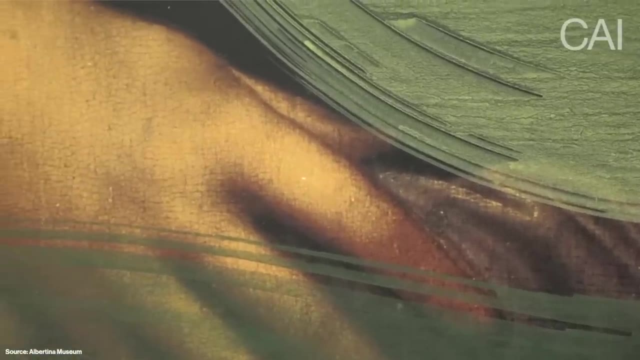 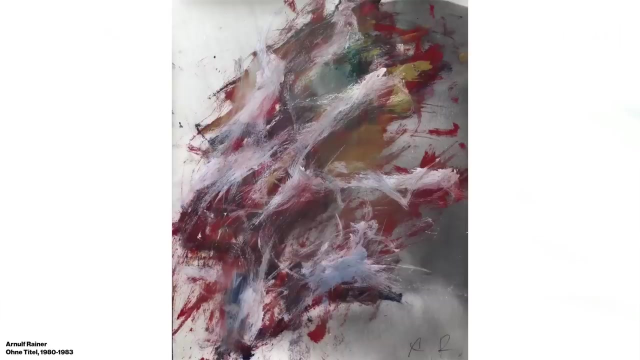 on top of them, Thick marks, layers of paint, gestural strokes and a connection with surrealism due to the implementation of automatism by painting with, for instance, a blindfold. The Austrian artist follows his instincts and urges working towards abstract tableaus and other experimental practices in his creative process. 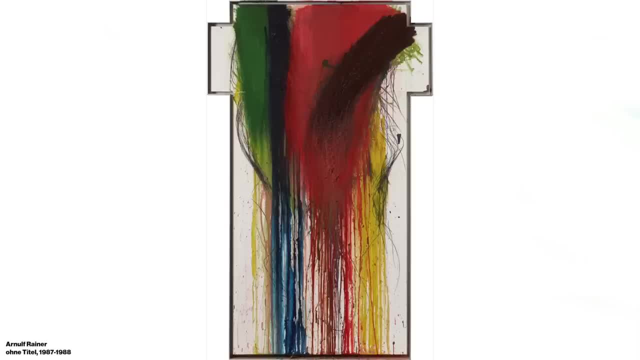 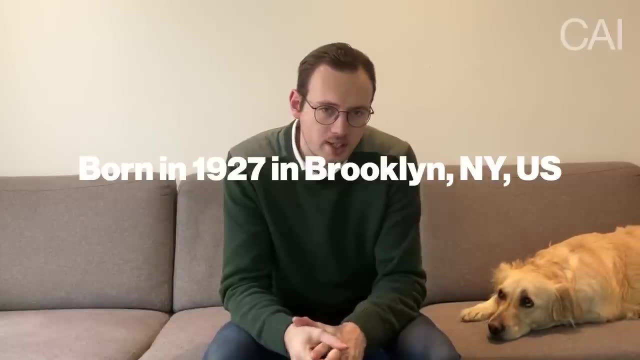 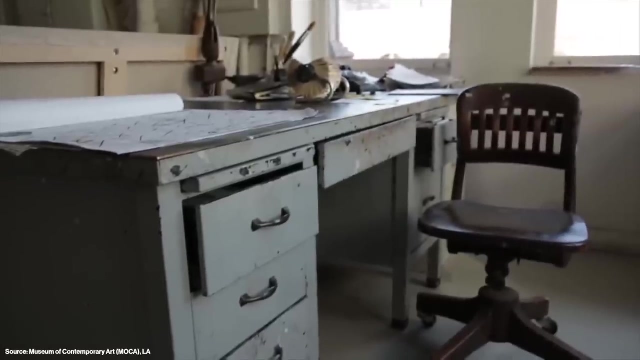 including the use of his feet or painting under the influence of drugs. Alex Katz, born in 1927 in Brooklyn, is an American painter, working and residing in New York City. Over the years, Katz has distinguished himself with a unique approach to figurative painting. Since the 1950s, Katz has dominated the art scene. 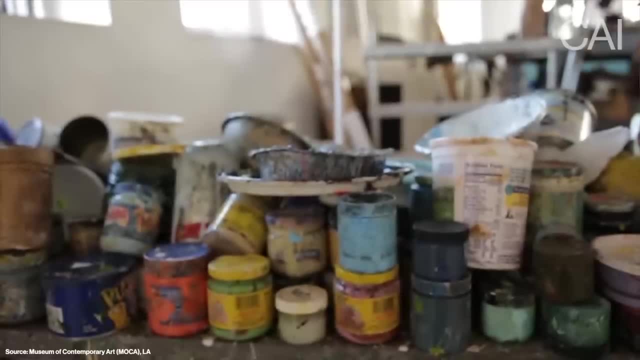 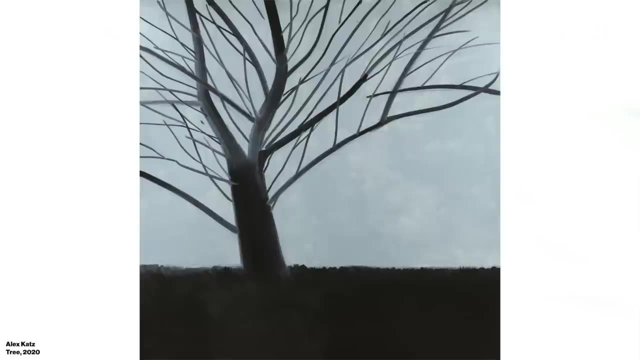 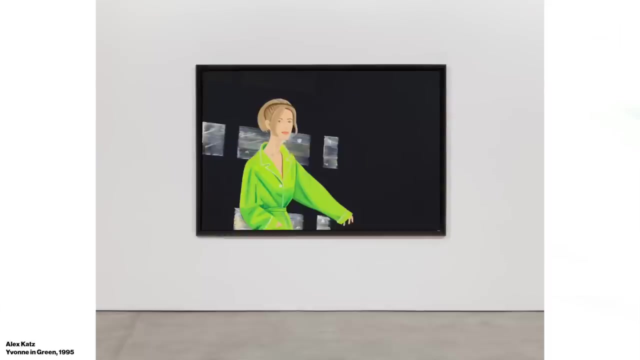 for seven decades. with his representational paintings of contemporary life, The American artist draws inspiration from films, advertising, friends and music, working primarily from life, Using large and flat planes of colour. Katz's figures are made out of flat shapes on a monochrome background, Using photographic techniques such as. 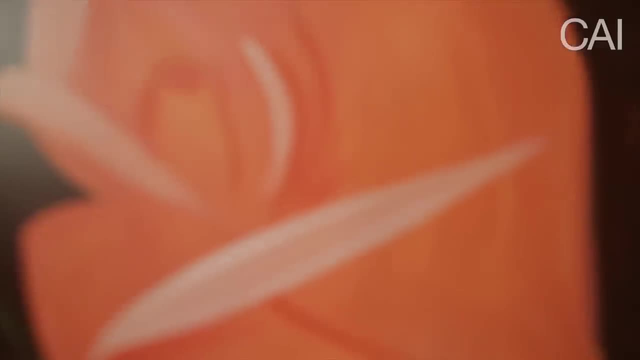 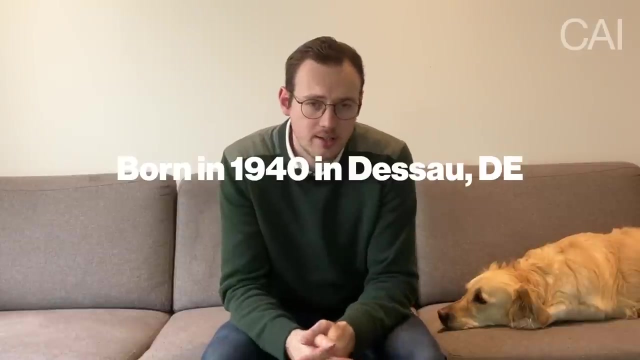 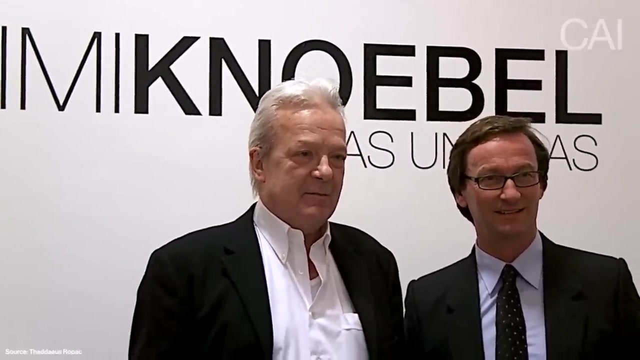 decoupage and cropping Katz searches for the perfect fragment of a figure to paint. Born in 1940 in Dessau, Germany, and currently residing and working in Düsseldorf, Imi Kneubel is best known as a painter. However, he incorporates drawing sculpture installation. 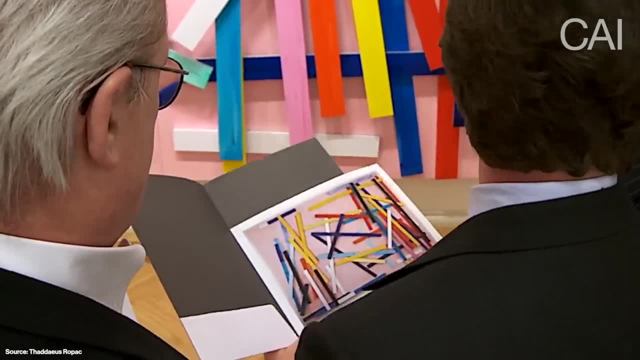 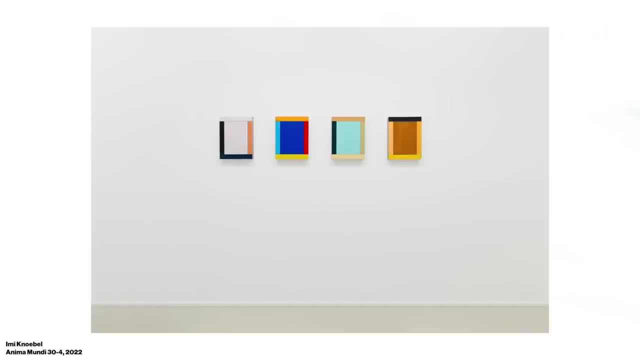 and even photography into his artistic practice. Kneubel discovered painting in the 1960s with a rigorous and basic approach of thick or thin vertical lines placed at variable distances from each other. Throughout the 70s, the German artist continued experimenting with his 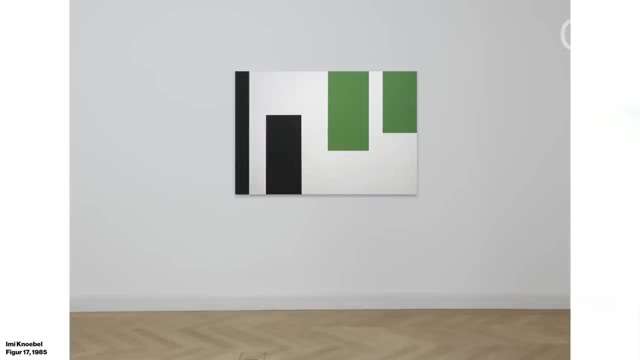 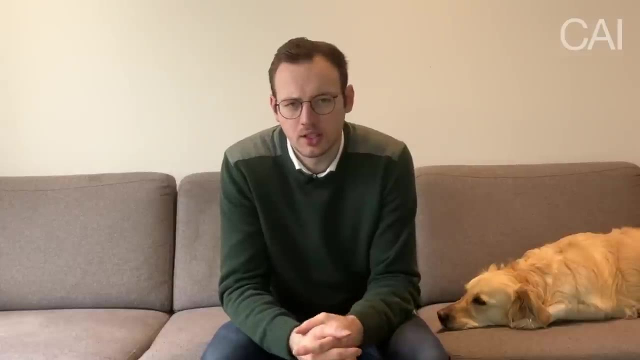 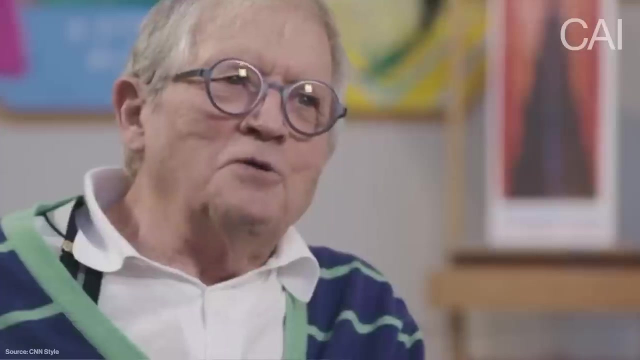 minimal approach, implementing projections, experimenting with colour and expansive painting. David Hockney. born in 1937 in Bradford, the UK, and currently residing and working in Normandy, France. Hockney has been adored for his work in the 19th and 20th centuries. He has been a great 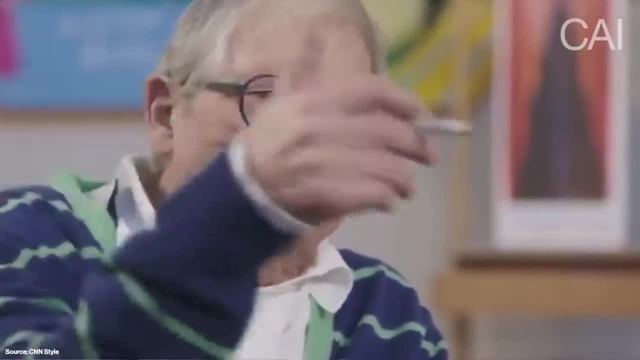 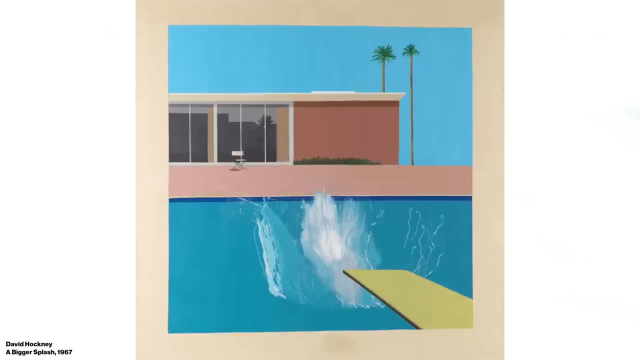 well-known protagonist for pop art, the British art scene and figurative painting in general. throughout the 20th century, Hockney continued to develop his distinctively painterly practice in the Hollywood Hills since the 1960s, where he lived and worked, translating his daily. 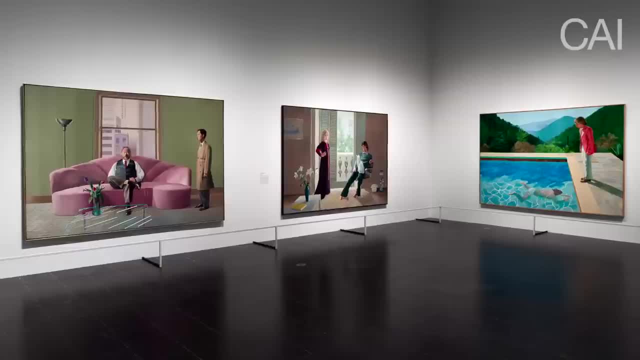 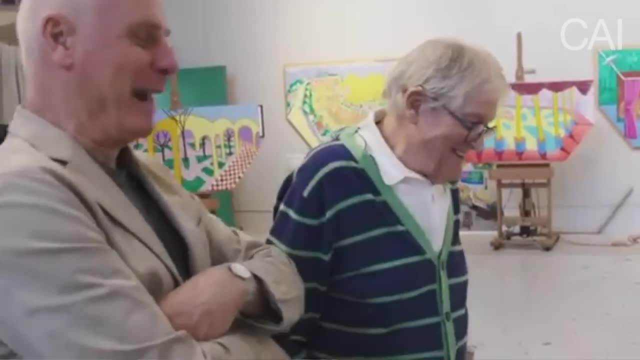 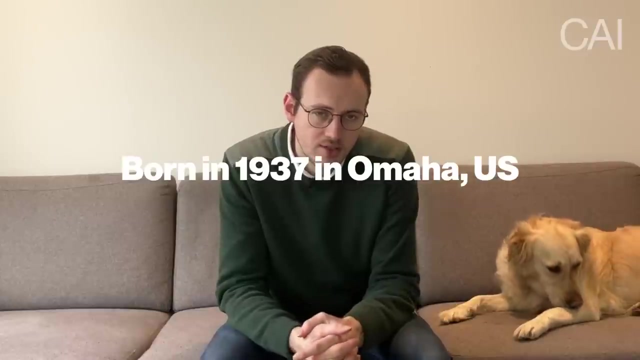 environment to his artistic practice. As a result, the exotic and sensual life by the pool in LA became visible in his paintings and the iconic British artist continues to work up to this day. David Hockney, born in 1937 in Omaha, the UK, is an American painter residing and working in. 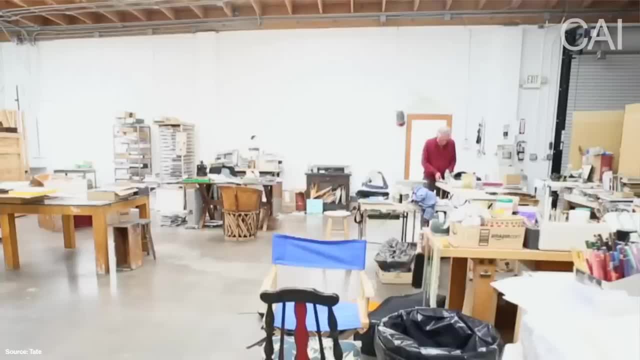 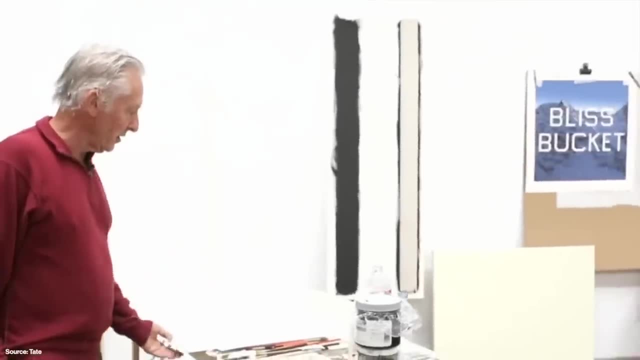 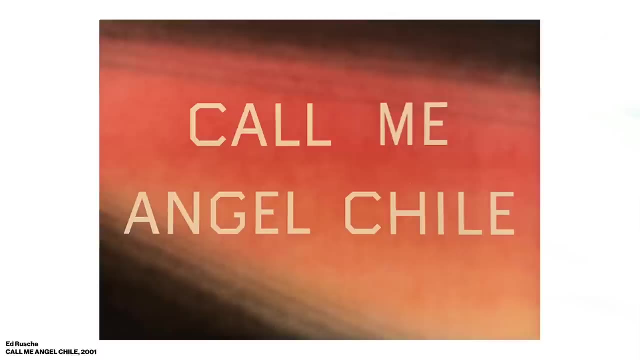 Culver City. Hockney is best known as the artist who abandoned the academic connotations associated with abstract expressionism and brought words to the universe of painting. Hockney uses words as forms, signs, materials and as subject matter to construct abstract pictures, Using humour and wit. 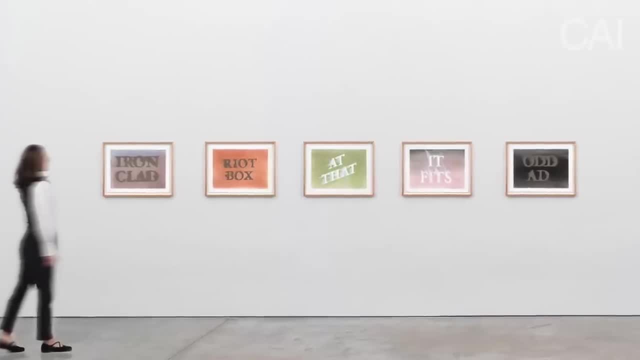 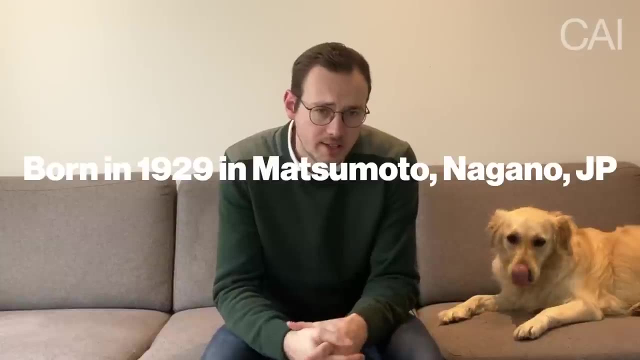 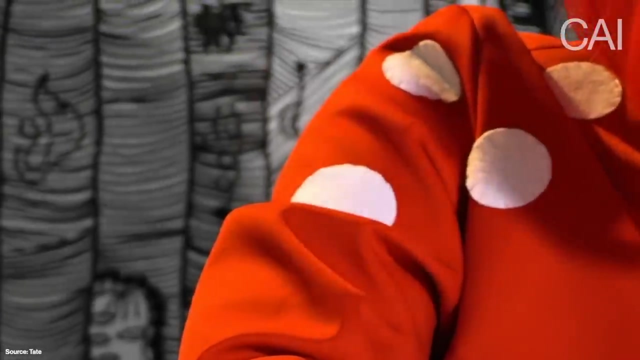 Hockney's word paintings achieved international praise as he intertwined the visual with language. Born in 1929 in Matsumoto, Nagano, Japan, and currently residing and working in Tokyo, Yaya Kusama is a contemporary artist best known for her unique and colourful paintings. 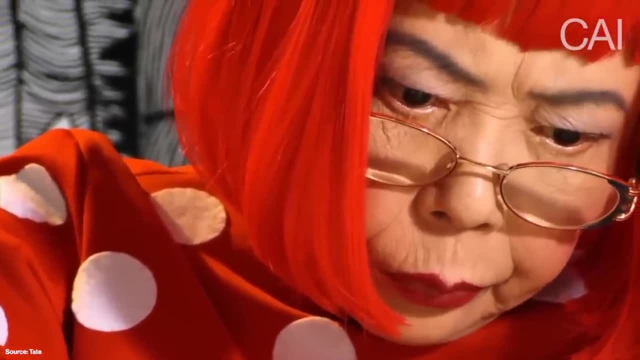 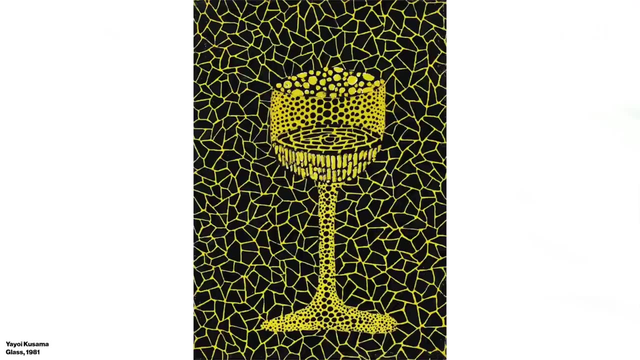 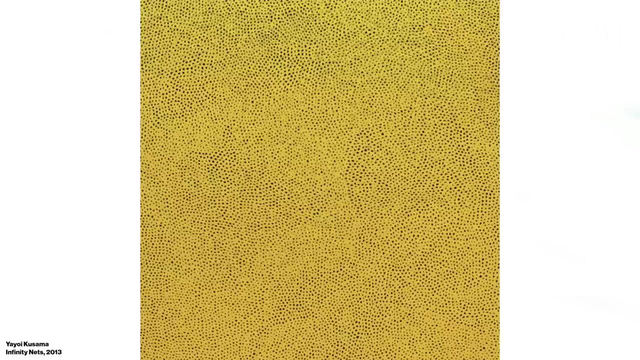 but also immersive installations and sculptures of pumpkins and polka dots. In the 1960s, with her paintings depicting ongoing loops and polka dots she called infinity nets, dazzling the viewer and combining figurative imagery with minimal abstraction in these mesmerizing organic patterns. 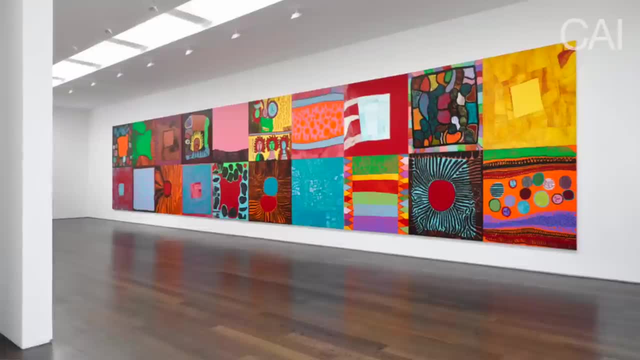 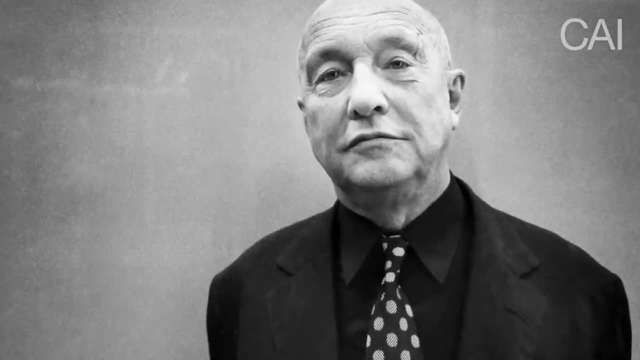 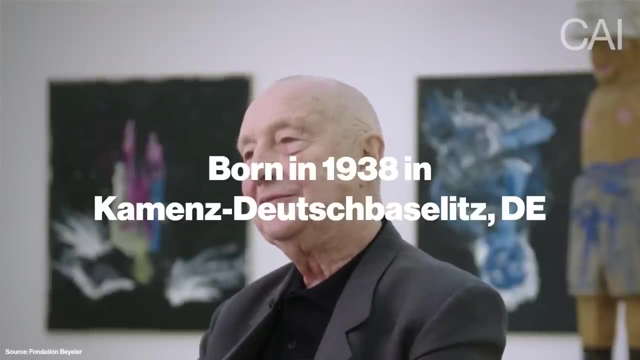 Kusama suffers from hallucination and aims to examine psychological aspects and autobiographical elements in her paintings. In second place, we have the illustrious career of Georg Baslitz. Born in 1938 in Kamenz-Deutsche Badslitz, Germany, Baslitz lives and works in Munich. 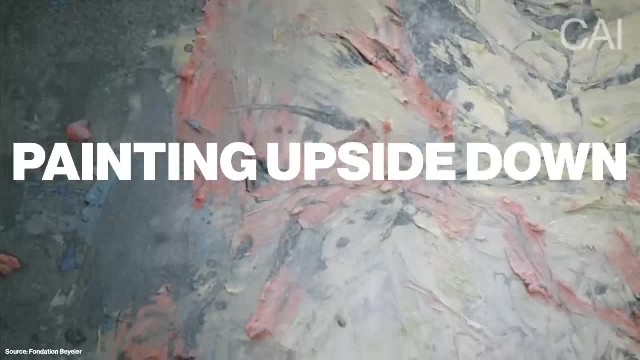 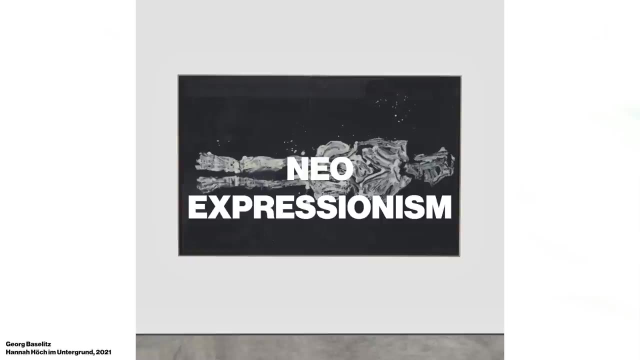 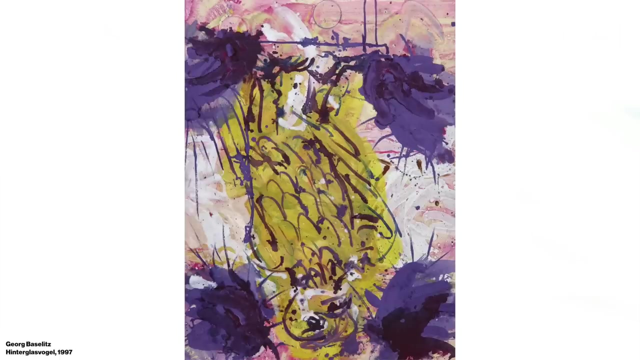 The painter is best known for his upside-down painted figures. He is one of the most important post-war artists and a pioneering protagonist of new European painting and neo-expressionism in Germany, rejecting the dominance of abstraction and painting representational elements. returning to the figure, The German painter, printmaker and sculptor. 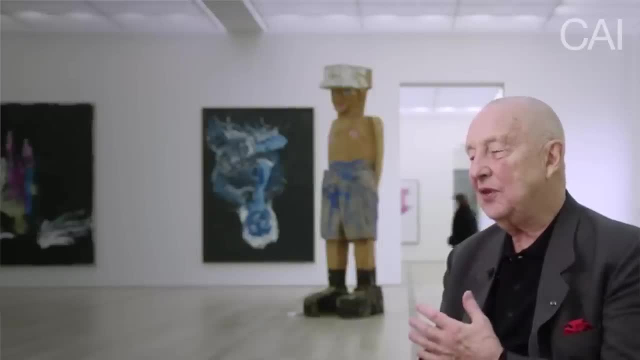 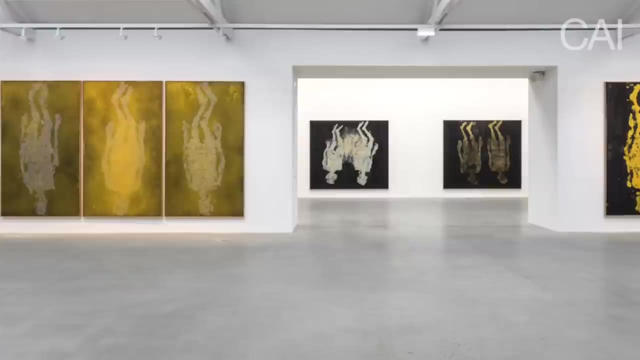 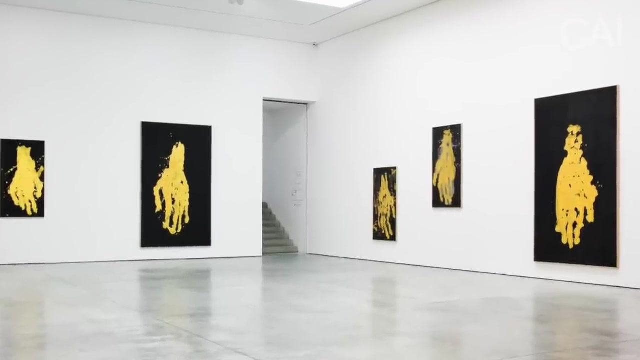 depicts his subjects upside-down to slow down the painterly process and the viewer's experience of the painting. In doing so, Baslitz achieves a unique balance of abstraction and figuration, depicting not only figures on their head but also landscapes, still-lives and more. 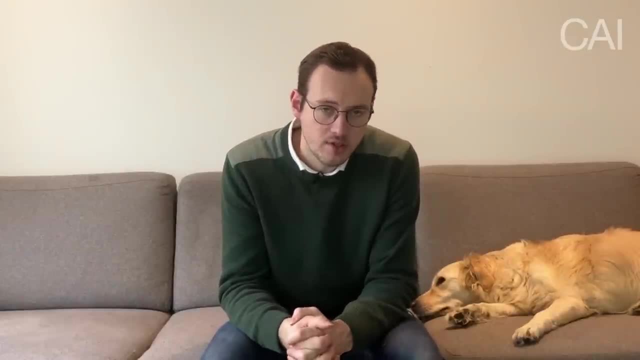 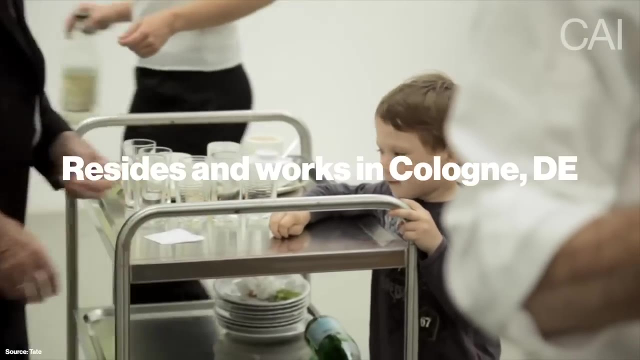 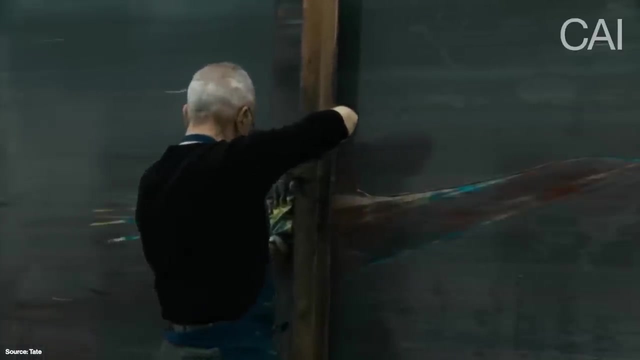 As last time, at the very top of our list as the most famous painter today we have Gerhard Richter, who in Dresden, Germany. Richter currently lives and works in Cologne. He dedicated his career to exploring the medium of painting in close relation to the effects of photography. 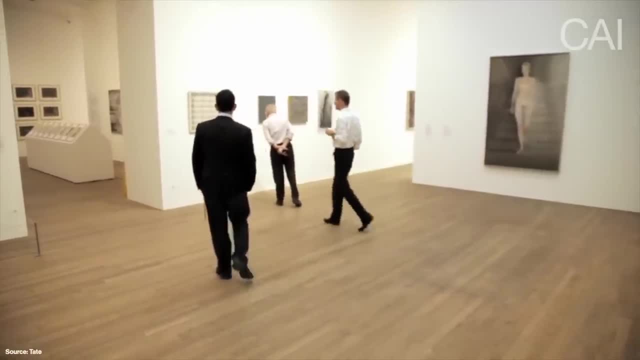 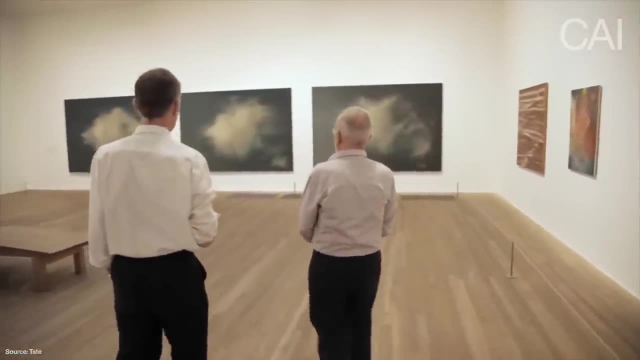 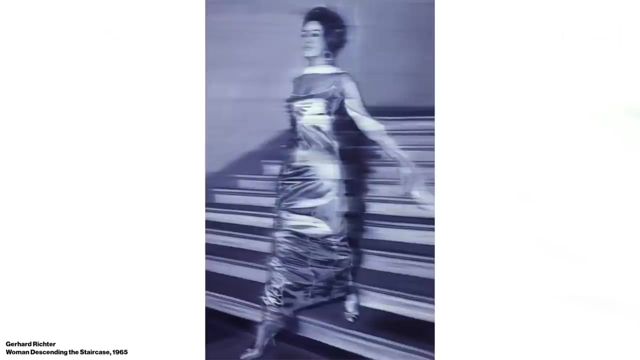 Richter achieved international recognition in the 1960s with his photo paintings. He rendered photographs into paintings varying in subject matter. think of landscapes, nudes, still-life painting, daily life, airplanes, alpines and more were painted with a. 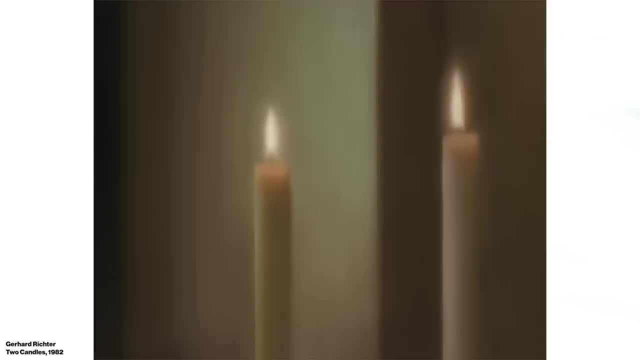 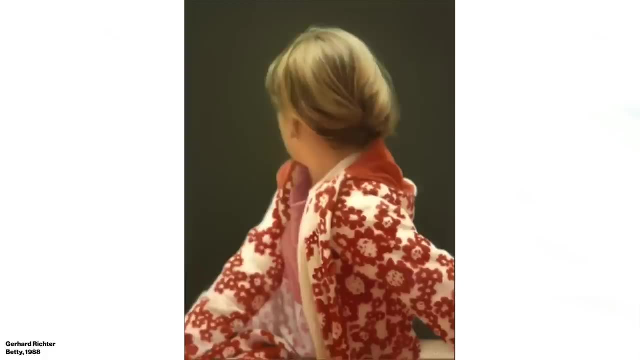 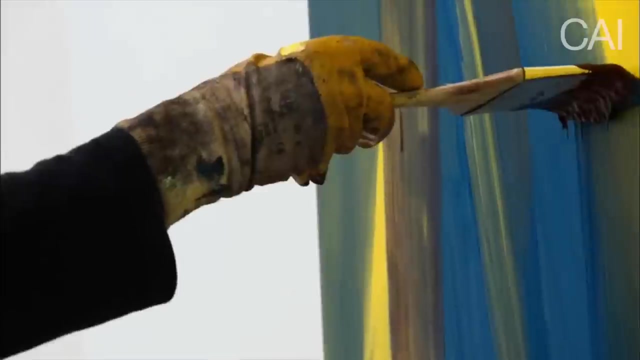 haste hovering over the photorealistic image, creating a blurred effect. This Richter blur or haste, introduced abstraction into his oeuvre, allowing Richter to move freely from photorealism to bold abstraction as no other artist has ever been able to do before. As we take on recent art history,